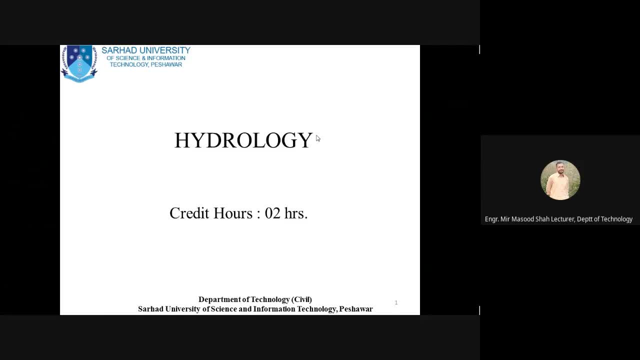 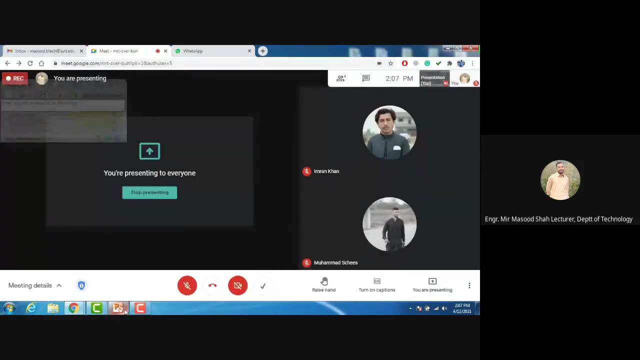 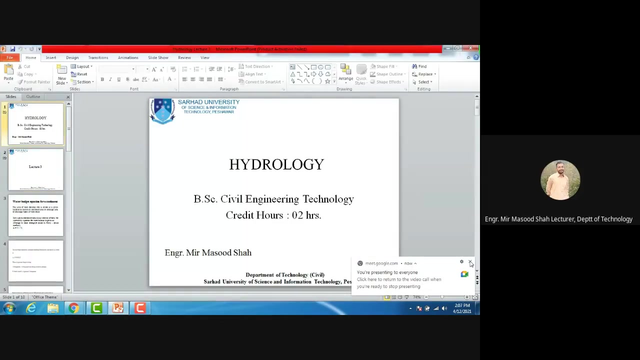 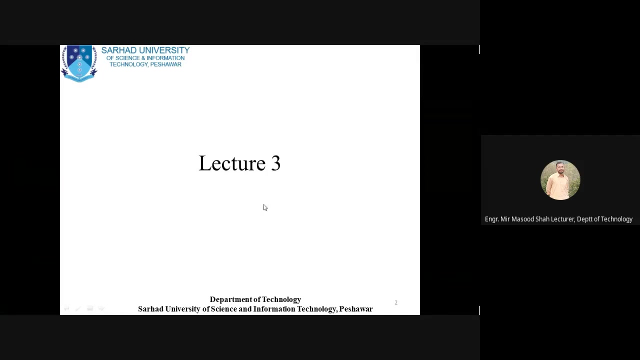 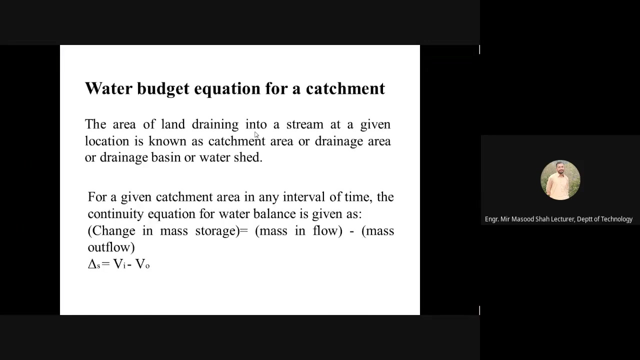 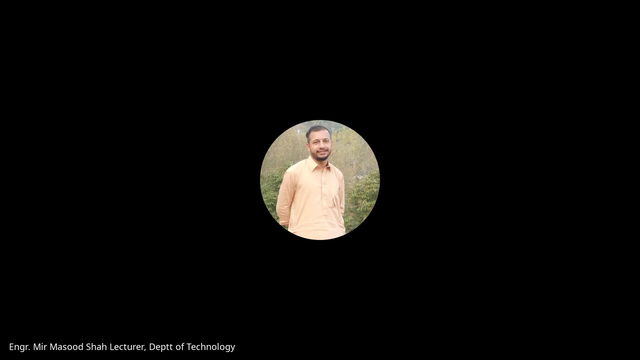 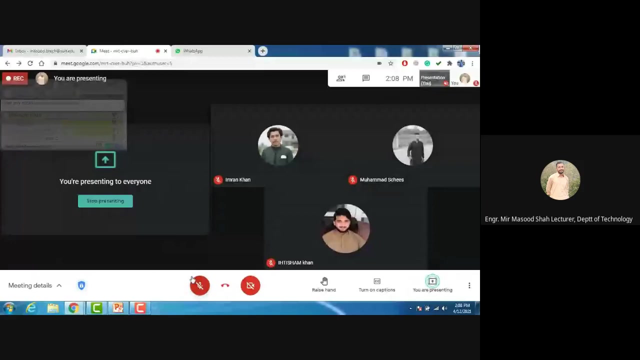 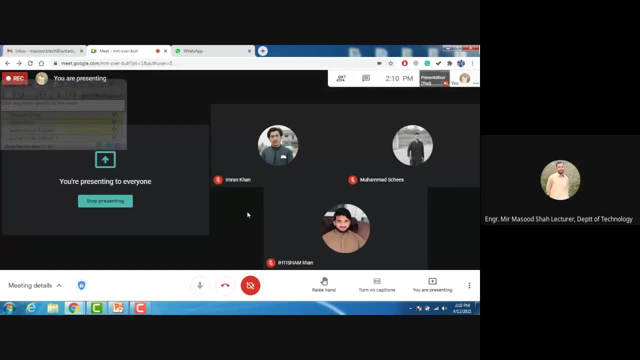 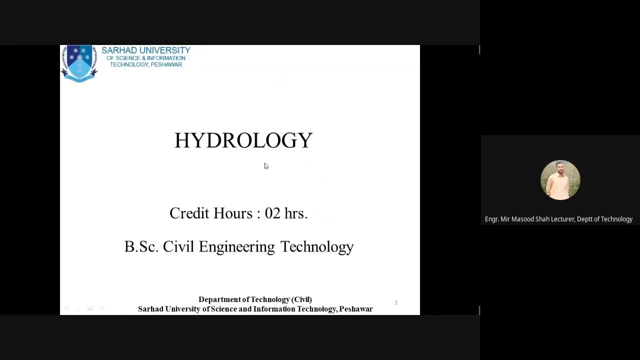 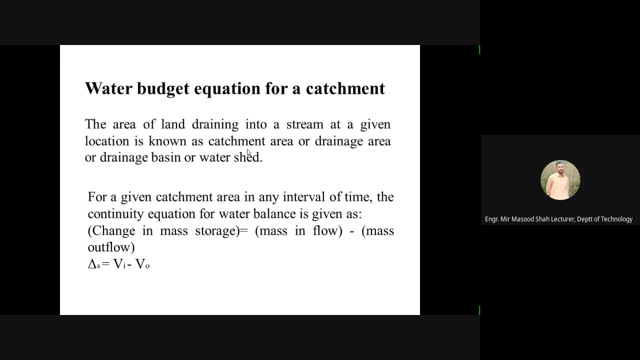 Thank you, Yes, Yes, Sorry, Sir, Sir, Sir. So our subject is hydrology and it is for BC Civil Engineering Technology, and the credit hour for this course is two hours. Today we will have lecture number three. In lecture number three, the topic we will study today is a water budget equation for. 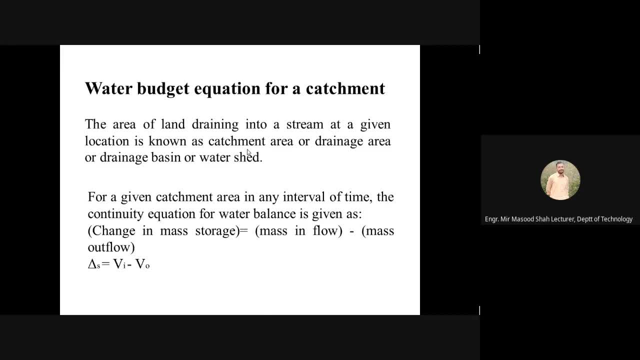 a catchment area. The area of land draining into a stream at a given location is known as catchment area or drainage area or drainage basin or watershed, So any area which drains into a stream at a given location, any location it may be. 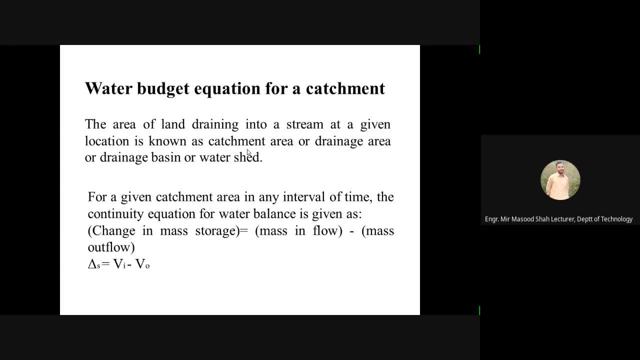 so it is that land area of land is known as the drainage area. It is also known as the drainage basin or watershed or drainage area For a given catchment area in any interval of time. the continuity equation for water balance is given as change in mass storage. that is equal to mass inflow minus mass outflow. 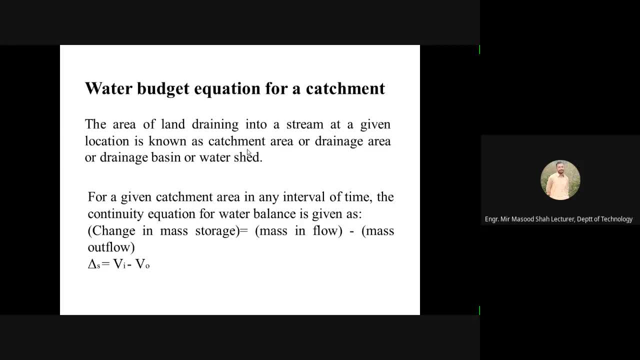 So, in order to get the continuity equation for water balance for a given catchment area in any time interval, 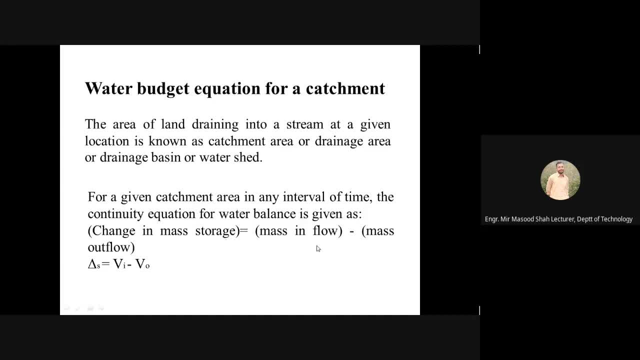 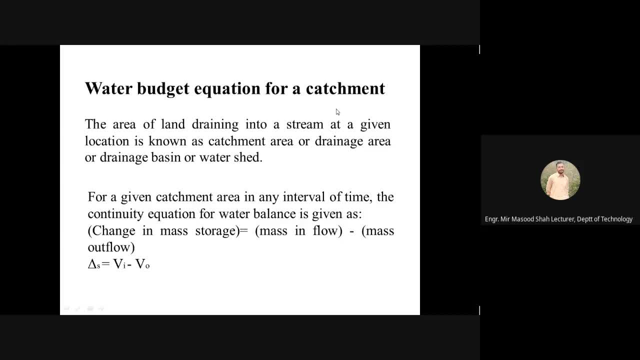 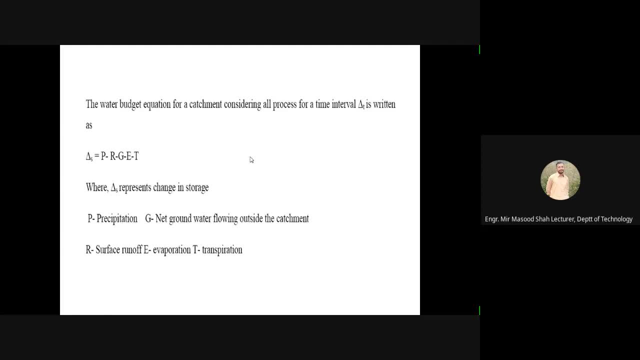 in storage may be expressed as: delta s is equal to delta s s plus delta s m plus delta s g, so in 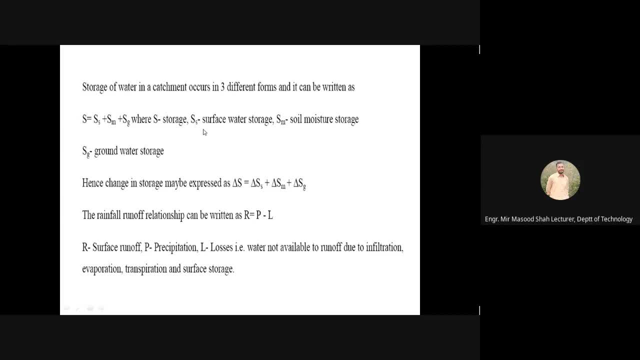 order to get the change in the storage uh. we denote uh- this uh above equation- as delta s equal to delta s s plus delta s m plus delta s g. the rainfall runoff relationship can be written as: r is equal to p minus s. this equation is used for finding uh the relationship between uh rainfall. 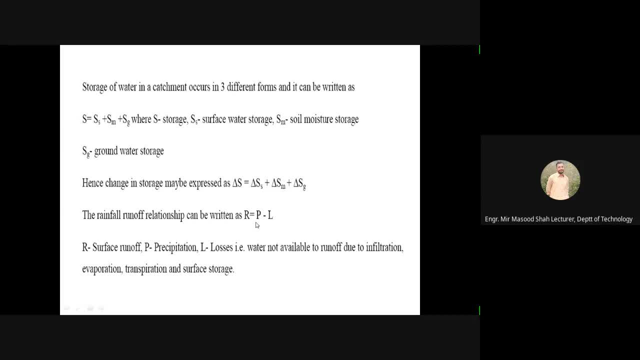 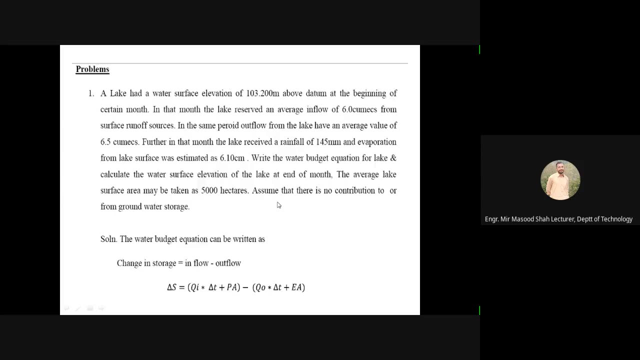 runoff. uh that in here, r is the uh surface runoff, p is the precipitation and l is the losses. that is, a water not available to runoff due to infiltration, evaporation, transpiration or surface storage. so uh, this is uh known as the water burgeoning equation for a given catchment area. 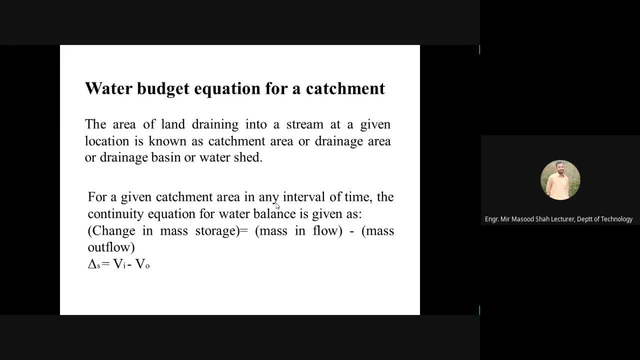 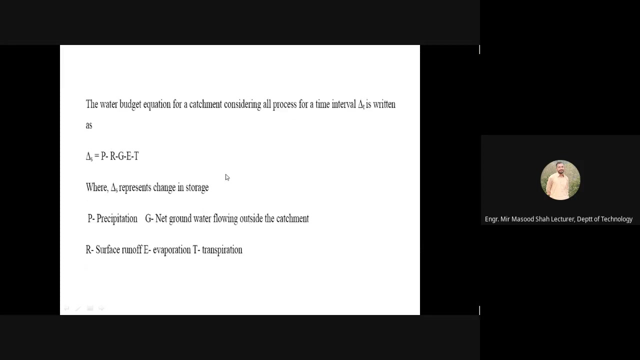 or also known as. This is the water balance equation for a given catchment area, Drainage area or watershed Drainage area or mass storage. change in mass: mass inflow, mass outflow. water budget equation considering all processes for a. 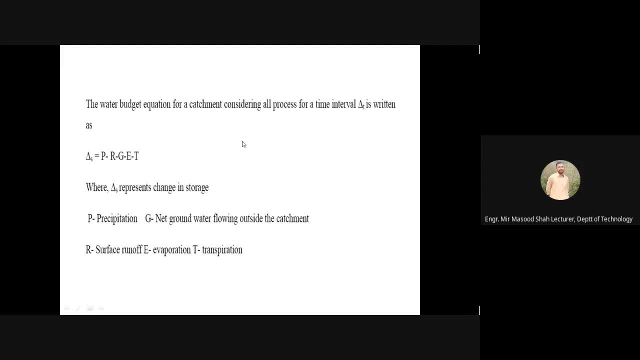 given time interval. delta T catchment area. delta S is equal to P minus R minus G, minus E minus T. P is net precipitation, R is surface runoff, G is net groundwater flowing outside the catchment area, E is evaporation. 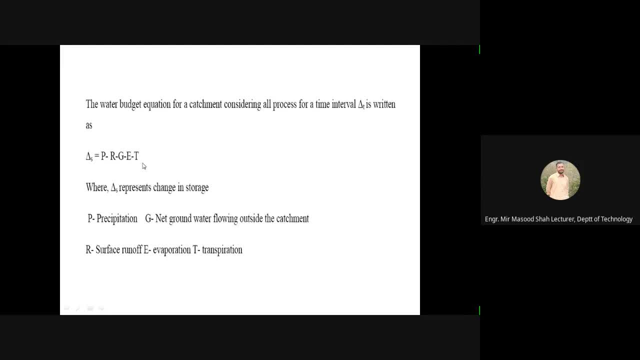 T is transpiration, Delta. S represents change in storage. The storage of water in any catchment has three different forms. S is equal to SS plus SM plus SG. S is equal to total storage. SS is surface water storage, SM is soil moisture storage. 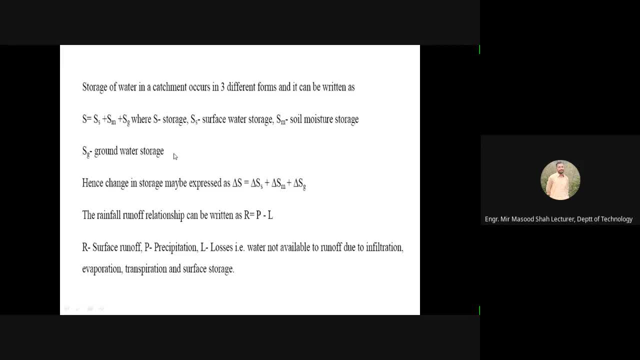 G is ground water storage. The change in storage is expressed as: delta S is equal to delta SS plus delta SM plus delta SG. What we call rainfall. R is equal to P minus L. R is surface runoff, G is precipitation, L is losses. 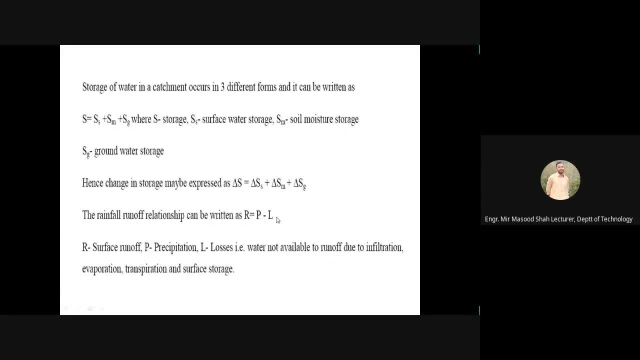 The losses occur when water that is not available. The process of water loss is called loss due to evaporation, transpiration or surface storage. There is no water loss in the soil. There is a loss of water. There is no water loss in the soil. 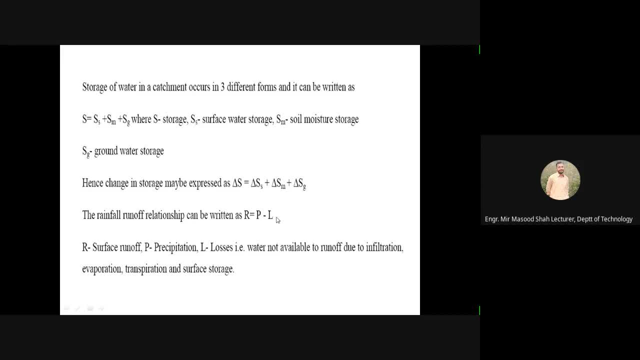 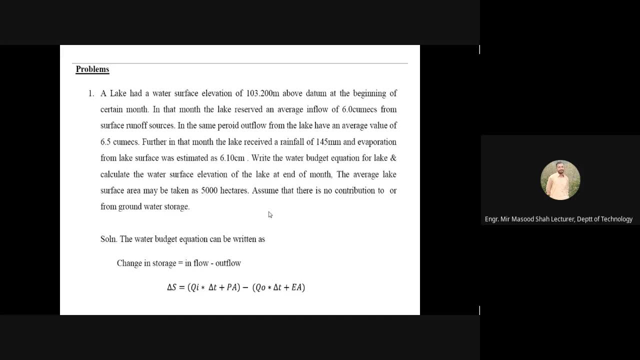 So we have problems. number one: a lake had a water surface elevation of 10103.200 meter above the datum at the beginning of certain month. in that month the lake reserved an average inflow of 6 cumecs from surface runoff sources. in the same period, outflow from the lake have 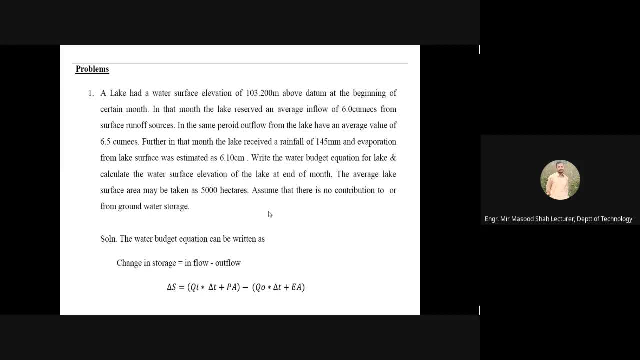 an average value of 6.5 cumecs. further in that month, the lake received a rainfall of 145 millimeter and evaporation from lake surface was estimated as 6.10 centimeter. write the water budget equation for lake and calculate the water surface elevation of the lake at. 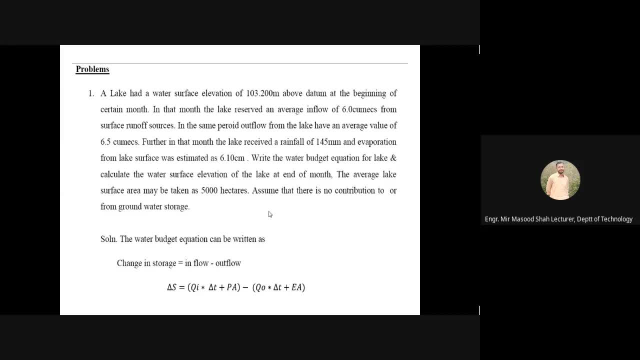 the end of the month. The average lake surface area may be taken as 500- 5000 hectares assume that there is no contribution to or from groundwater storage. So in this problem we will calculate the water surface elevation of the lake at the end of the 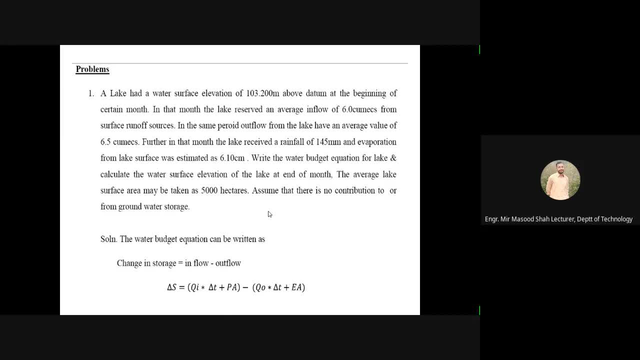 month. also, we will write the water budget equation for the lake. the given data is the water surface elevation is given, which is 103.200 meter. So in the data we will write, the water surface elevation is equal to state average 6, 60 AM. 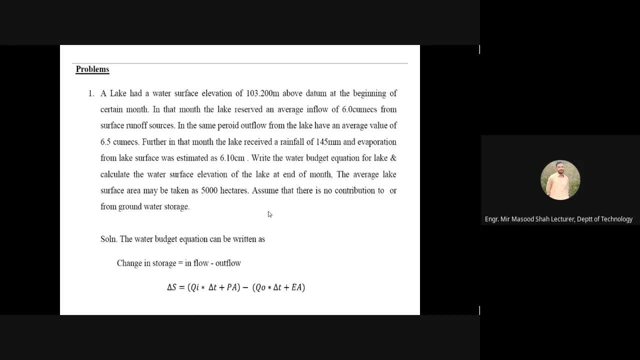 in 2000, with befitting movement of water, surface elevation is 1017 và poryuk j 3.007 meter above the Datum in the beginning of a certain month. Ourцо The lake reserved average inflow is given, which is six cubic, that is, six cubic. 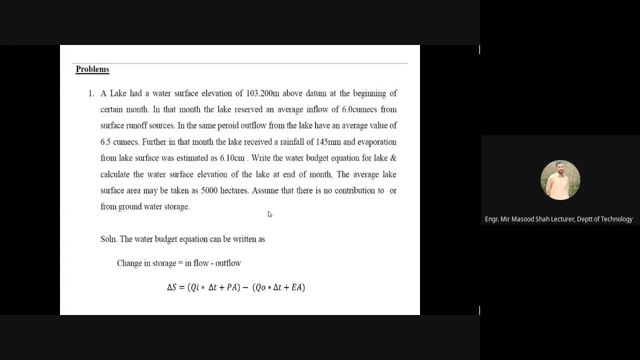 meters per second from surface runoff sources. Also in the same period, the outflow from lake have an average value of 6.5 cubic, that is, six 2500 cubic meter per second In that month. further by lake receive 145 millimeter of rainfall. So that with 6 m per second in that same period we 음악 also average inflow values, are establishing 6.5 cubic meter per second in that month, The upper ndersonal walls core area of 6 meters per second and at the second, depending on the and Tonestine. 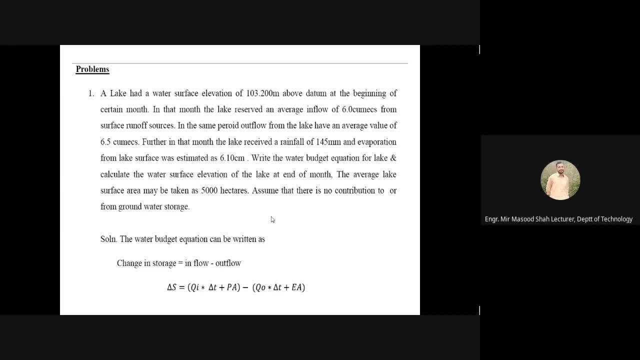 rainfall and uh. in that period the operation from the lake surface was estimated to 6.10 centimeter. the average surface area to be taken for the lack lake is 5000 hectares. we have to assume that there is no contribution to or from groundwater storage. 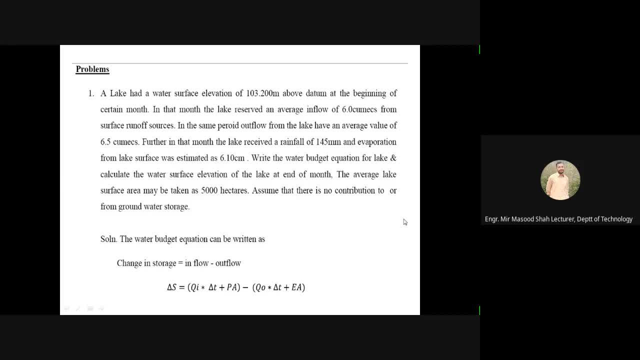 so, uh, first of all we will write the water budget equation, uh, and it can be written as: change in storage is equal to inflow minus outflow, so change in storage is denoted by delta s inflow. is q i into delta t plus p? into a minus q? naught into delta t plus e a. 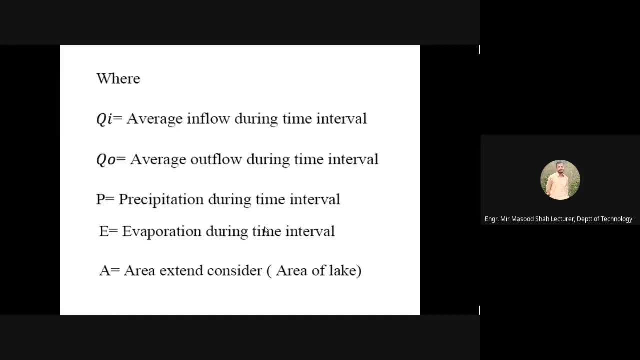 means, that is: q. i is the average inflow during the time interval, q. naught is the average outflow during the time interval, p is the precipitation during time interval, e is the evaporation uh during time interval and a is the extended area. extend uh standard. 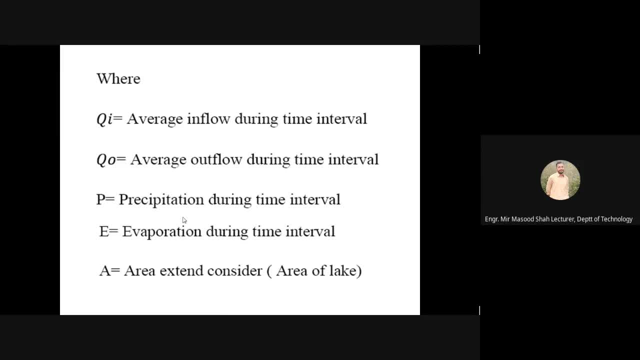 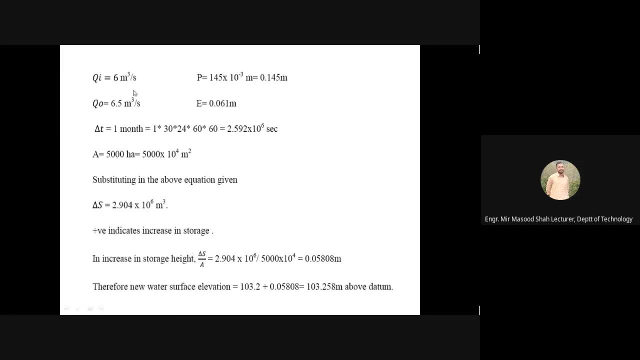 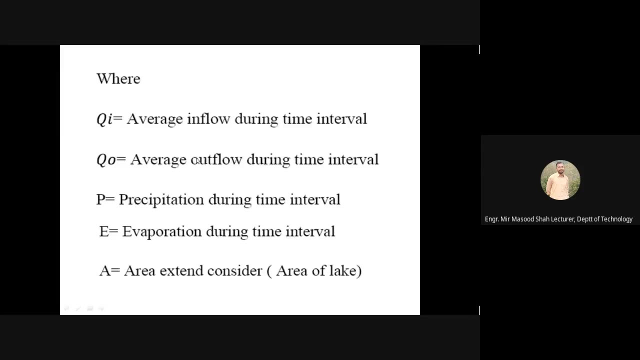 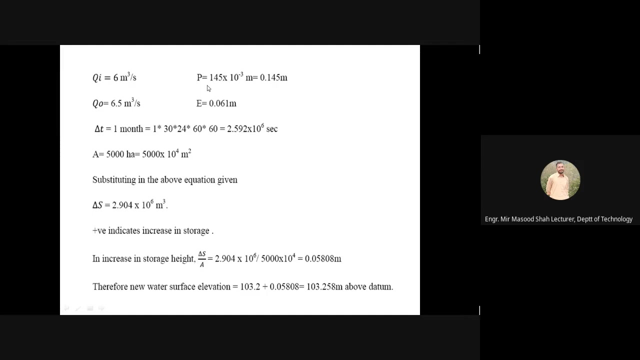 consider that is area of the leg. so these are the different terms, uh, which are explained here. uh, so q, i, which is the uh average inflow during the time interval is given, that is uh six qubits, that is, six cubic meter per second. uh p date is the average. uh, sorry, the rainfall that is received during that month is 1: 45. 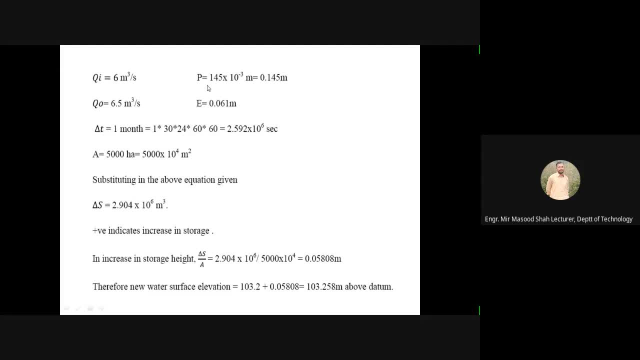 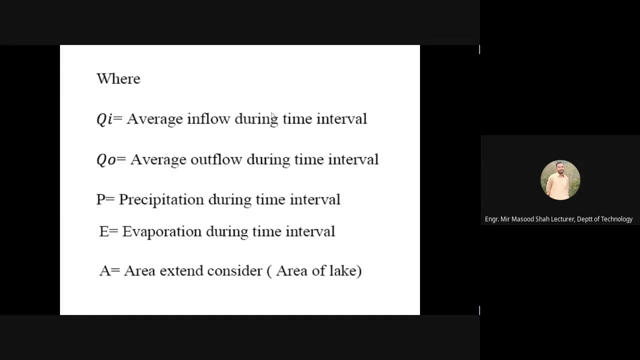 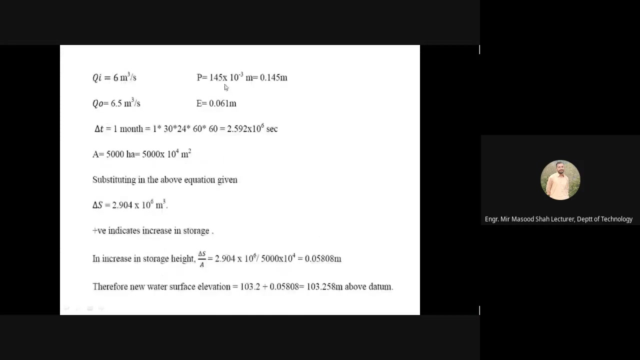 centimeter. so, uh, that is equal to 0.145 meter. 145 centimeter is equal to 0.145. in fact that is a millimeter. sorry, i told that it is 0.145 145 centimeter. it is 145 millimeter, so 145 millimeter is equal to 0.145 meter. q naught. 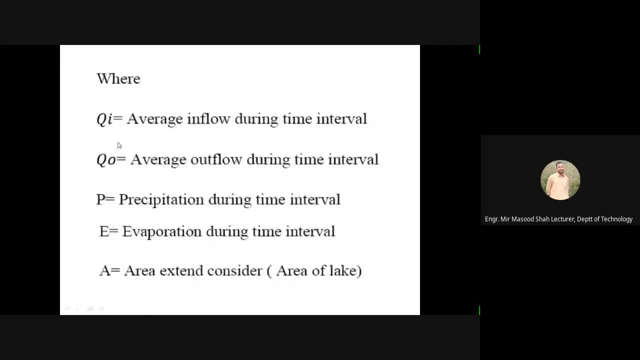 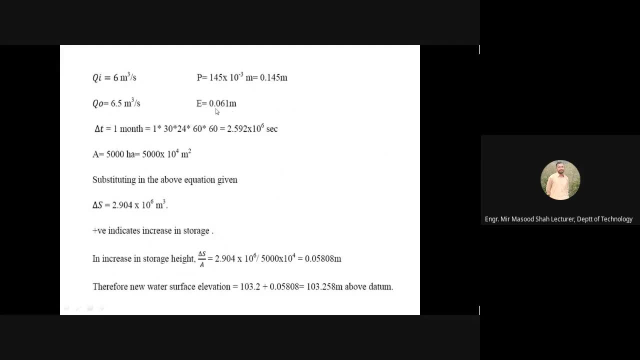 is the average outflow during the time interval and that is equal to 6.5 cubic meter per second. which is given is the evaporation uh from the leg that is given, which is 6.1 cent millimeter, and that is equal to 0.061 meter. delta t is one month, so that is 1 into 30. one month they have 30. 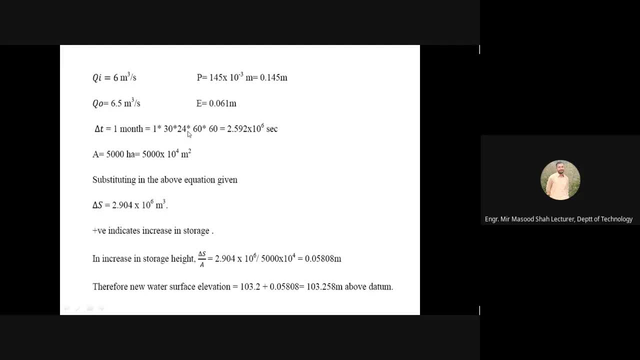 days, uh, and one day have uh. one day is uh 24 hours and then one hour is 60 minutes, uh, and 60 minute have 60 seconds. so we will get the total delta t. that is the time in, that is in second. that is 2.59. 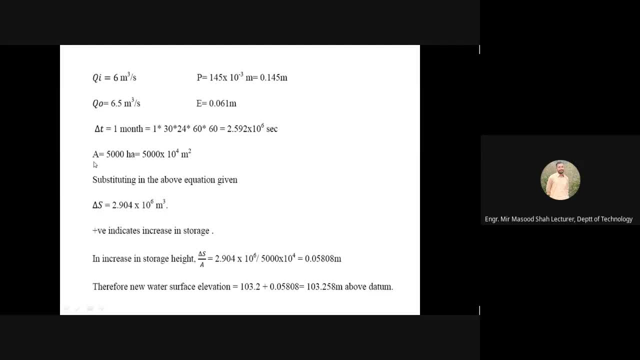 into 10 is power. 6 seconds. the. a total area a is equal to 5000 hectares. that is equal to 5000 into 10 is to our 4 square centimeter. now substituting the values in the above equation, so we will get: 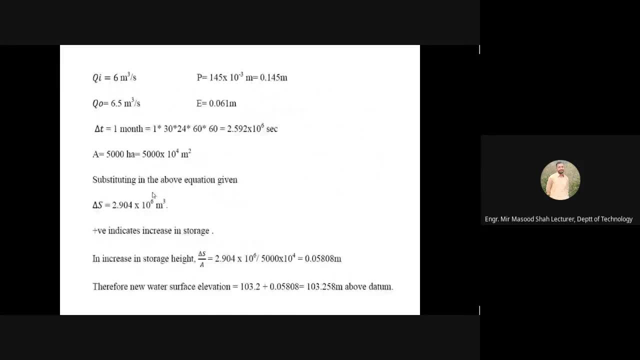 the total uh change in storage delta s that is equal to uh 2.904 into 10 is power 6 cubic meter. the positive sign uh in the positive value indicates that the uh increase in storage, that we uh have an increase in the storage water in in. uh in increase in. 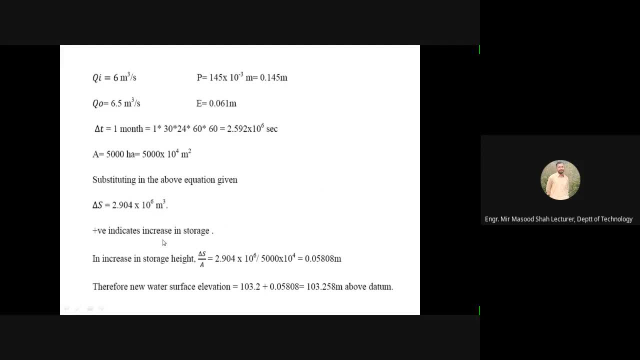 storage height. delta s, divided by a, is equal to 2.904. into 10 is power 6 divided by 5000 units, power 4 is equal to 0.05808. so this much a height. uh, uh, uh, a total change in height. 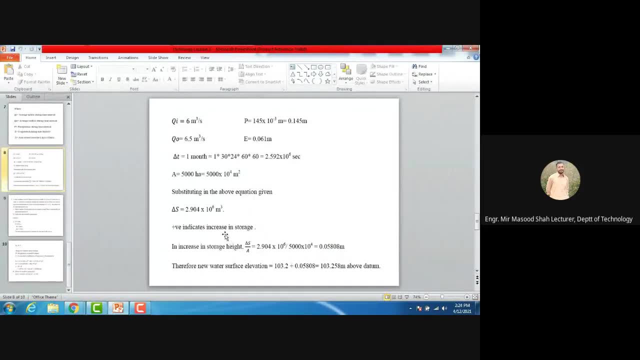 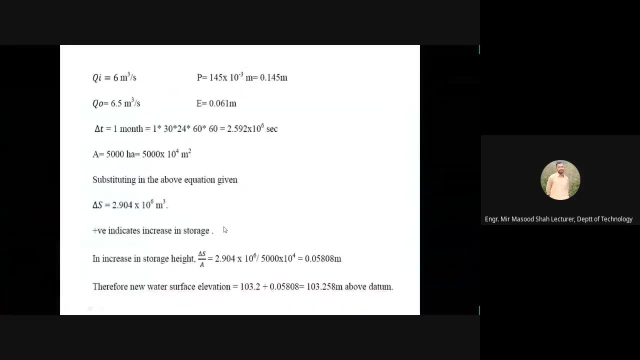 uh, uh, uh, uh uh uh. surface water elevation. in order to calculate the new surface elevation, the given surface elevation is 103.200 meter, so add 0.05808 with this value and you will get the new water surface elevation, and that is equal to 103.258 meters above the data. so in this way you will. 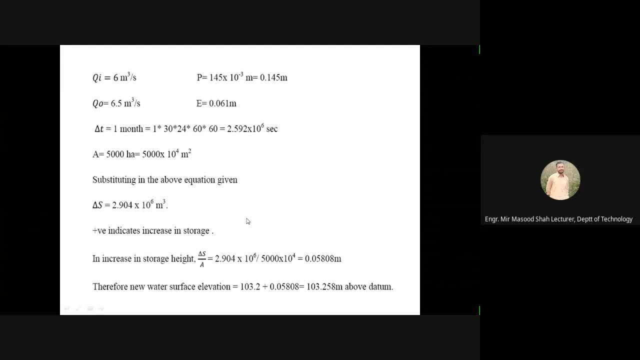 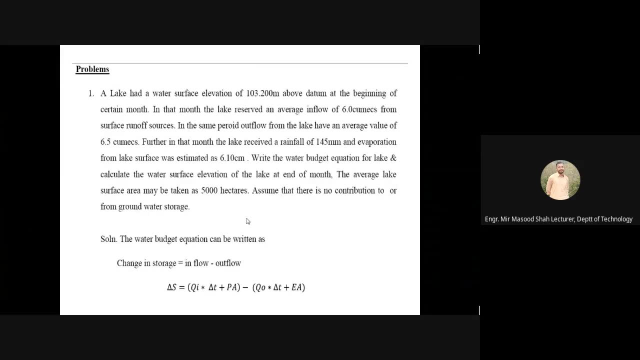 calculate the total new surface elevation and also the write the water budget equation for a given leg is the problem can have your part to have what elevation you have given. here we like have a studio, have water saturation given energy: 103.2 meter above the data in. 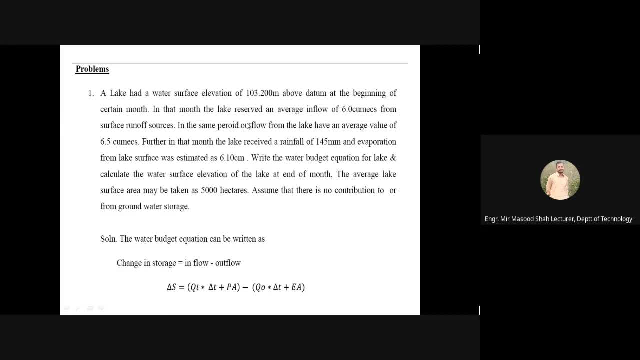 the beginning of the month we be certain month here. your leg carries under your reserve average. in flow have a six cubic meter per second here, or just from surface run of sources here, or your outflow: here we have a six point five cubic meter per second here. 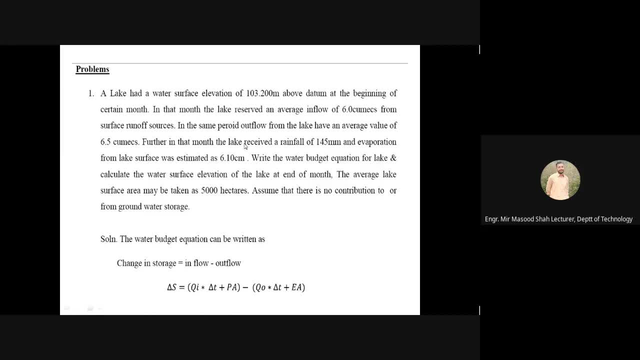 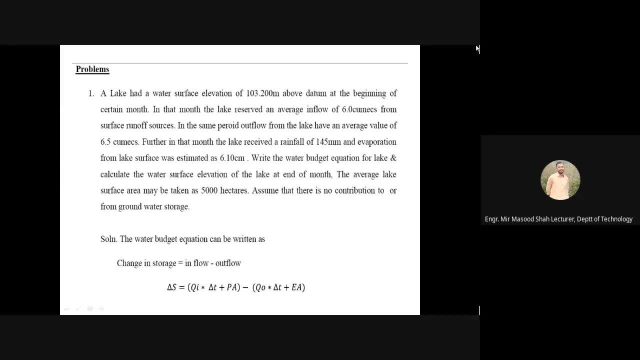 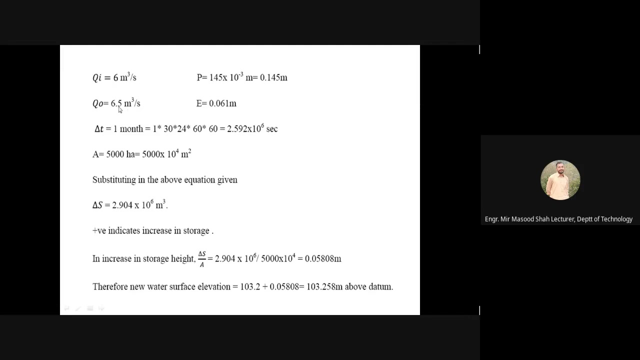 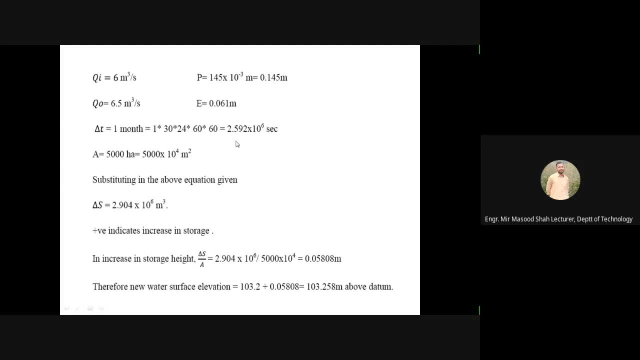 meter. time: 2.592 Newton's power, 6 seconds. area: 5000 Newton's power- 4 square meter. So we will get the total delta S value that is equal to 2.904 in terms power: 6 cubic meter per second. 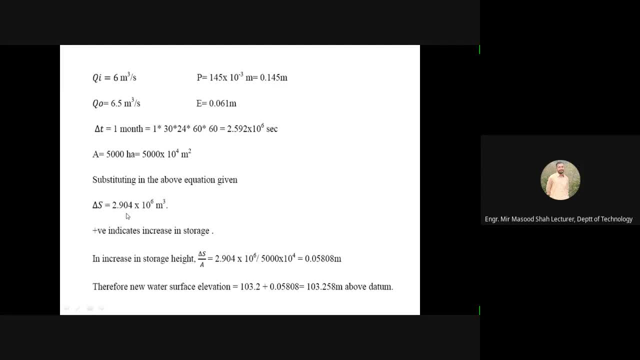 So we will get the increase in storage height. so what we have is 0.05808 meters. okay, So, given the water surface elevation above the datum line, you will get the new water surface elevation, and that is equal to 103.258 meters above the datum. 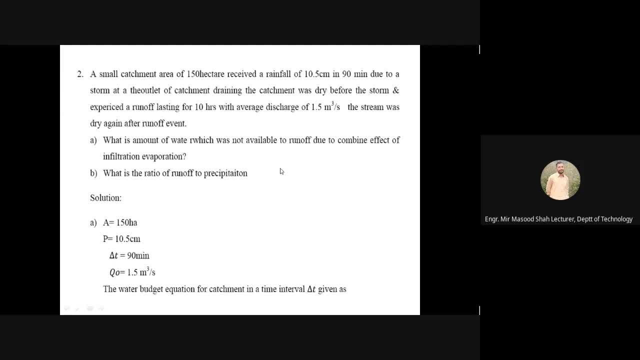 The next example is a statement of. the example is a small catchment area of 150 hectare received a rain fall of 10.5 centimeter in 90 minutes due to a storm at the outlet of a catchment training. The catchment was right before the storm and experienced a runoff lasting for 10 hours with average discharge of 1.5 cubic meters per second. 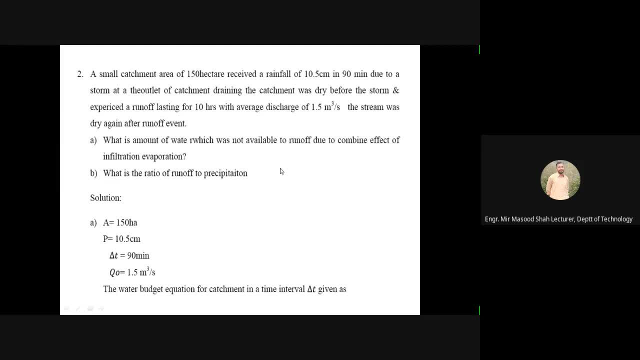 The stream was dry again after runoff. What is the amount of water which was not available for a runoff, which was not available to runoff due to combined water? So we will get the total delta S value that is equal to 2.904 meters per second. 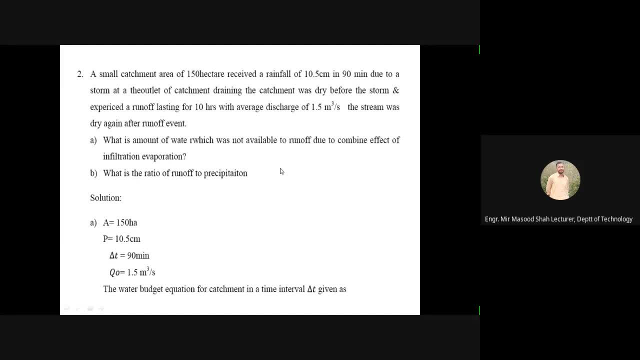 So in this example we will have to calculate the amount of water which is, was not available to runoff are due to combine effect of infiltration, evaporated. So in this example we have to calculate the amount of water which is, was not available to runoff due to combined effect of infiltration evaporated. 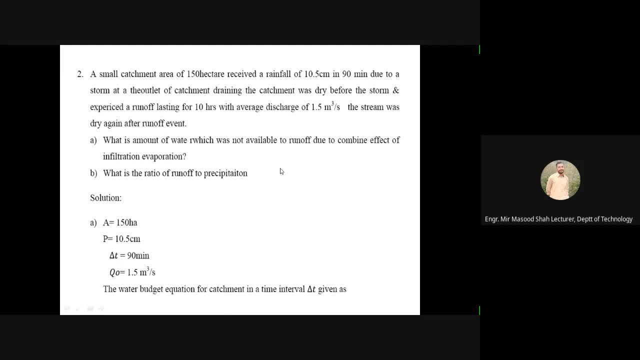 Also we will have to calculate the ratio of runoff to precipitation. The given area values are: the catchment area is given, which is 150 hectares. rainfall, which is 150 hectares. received uh is given 10.5 centimeter at the time is given 90 minutes. uh also, uh, the uh. 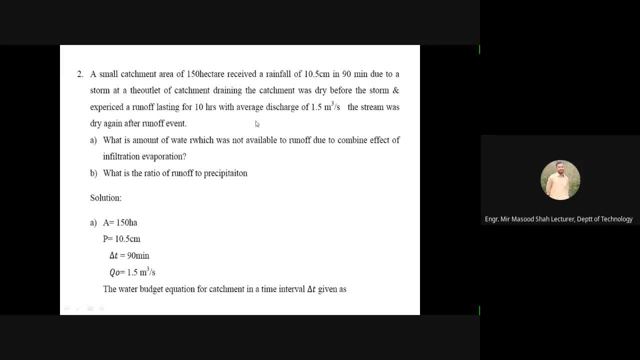 runoff is given which is uh, lasting for 10 hours lasting uh, uh, and the stream was dry again after the runoff event, rightly after the event of runoff. so, solution and solution: we will write the given data in given data. we have area given which is 150 hectares. precipitation is given: 10.5 centimeter delta t. 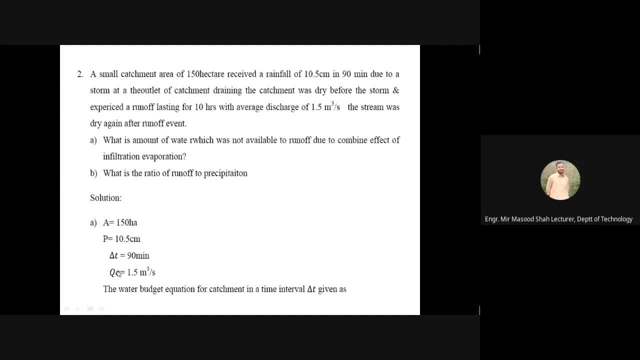 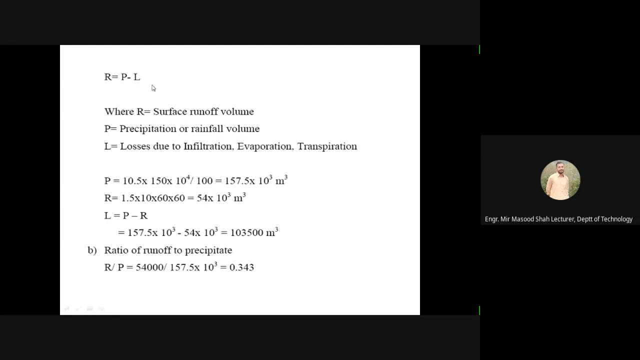 that is, time is given 90 minutes, uh outflow is given and that is 1.5 cubic meter per second. the water budget equation for a catchment area in a time interval, delta t, is given, as r is equal to p minus l. here r is: 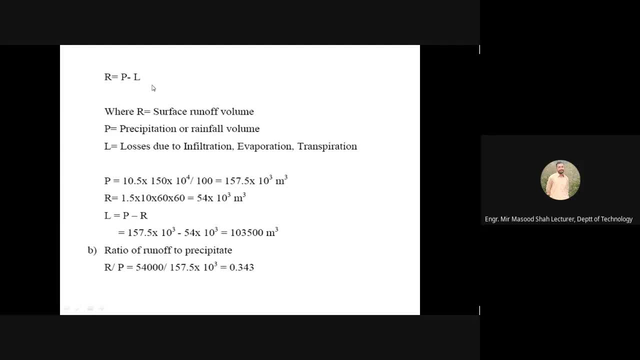 the precipitation, rainfall volume and lsd losses due to infiltration of operation and transpiration. here p is uh, the total uh precipitation. that is 10.5 into 150, into 10, to the power 4 divided by 100. uh. so 10.5 divided by 100. 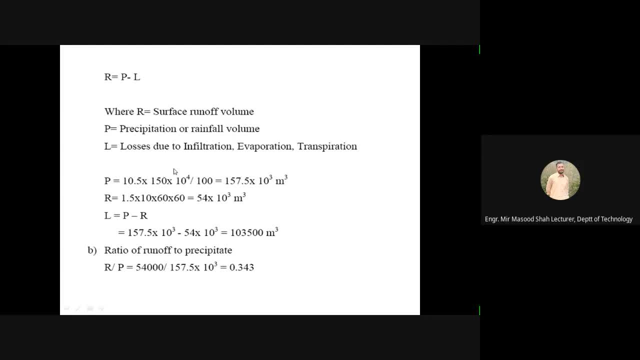 so you will get the total net precipitation, uh, or rainfall volume, that is 157.5, into 10 power mine attendance, power, three cubic meter. this much amount of rainfall is the occur and this is the total volume of the precipitation or rainfall water, uh, the losses are. 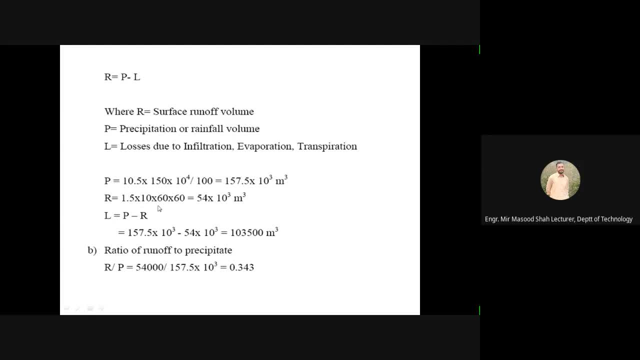 is uh, uh, sorry. the surface runoff r is equal to 1.5 into 10, into 60, into 60. uh, here, the total runoff is, uh, 1.5 cubic meter per second. so, uh, the time, uh, here, multiply this value, uh, with the time, that is 10 hours. 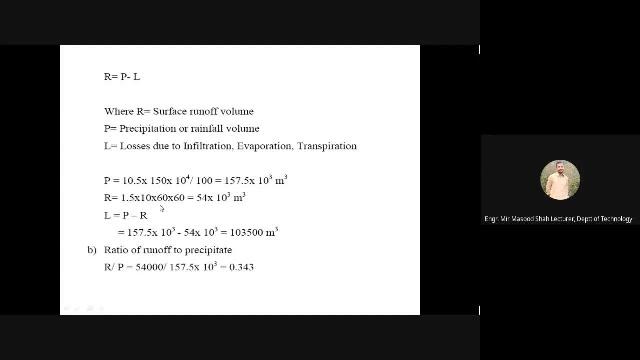 multiplied this with 60 uh minutes- one hour i have 60 minutes and also one minute has a 60 seconds, so you will get the total uh surface runoff in cubic meters, that is 54 into 10 inch power: 3 cubic meters. so in order to calculate the losses due to infiltration and evaporation, we will get l is. 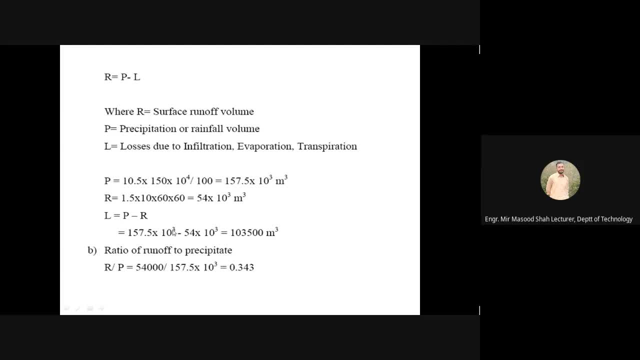 equal to p minus r. subtract the total uh precipitation of- uh, sorry, the total uh around the surface runoff from the precipitation and we will get the total losses due to infiltration operation and transpiration. so, uh, the total value of p is 157.5 into 10 power minus 3, 10 power 3. 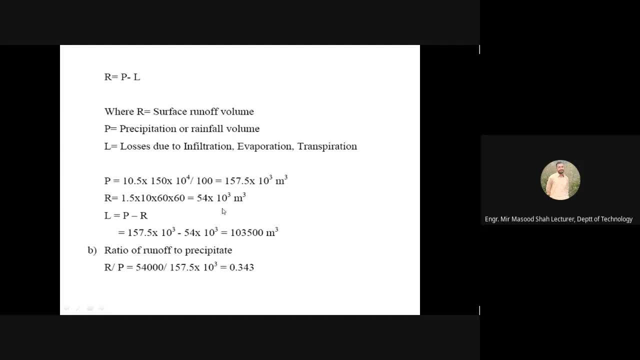 minus r, that is 54, into 10 power 3, so we will get the total losses due to infiltration and evaporation that is 10, 35 0, 0 cubic meter. so this much uh losses occur due to infiltration, evaporation during the process and now in uh. in the second case we will find the 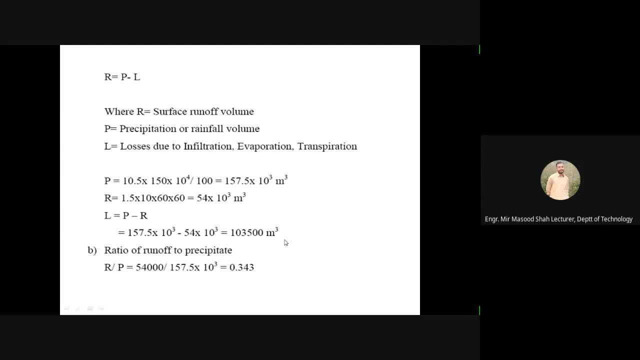 ratio of the runoff to precipitation. so in order to find the runoff to the ratio of runoff to precipitation, we uh, we have: r divided by p, r is equal to uh 54 000 and a precipitation is 157.5 in the trainer's power, uh three. so the total ratio of runoff to precipitation is: 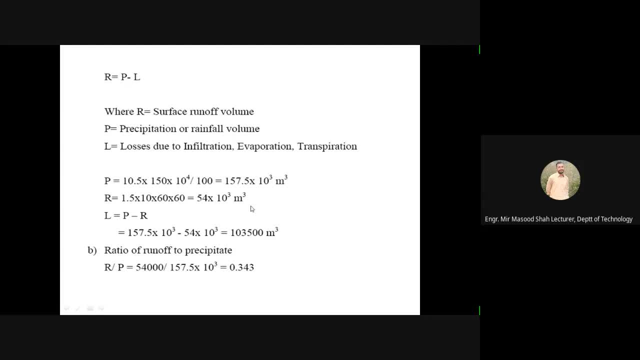 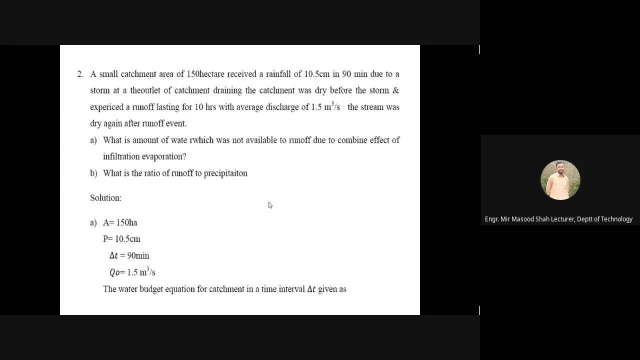 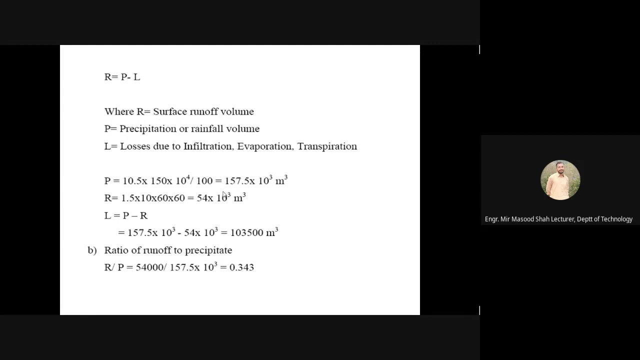 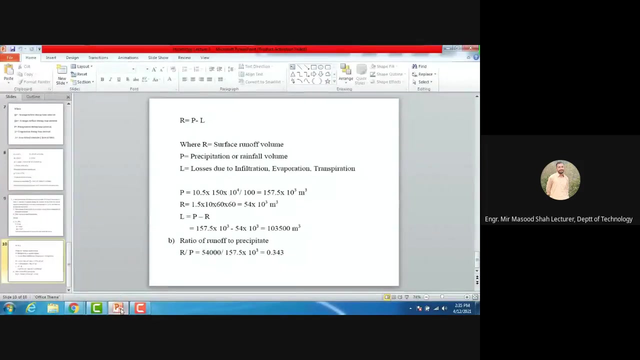 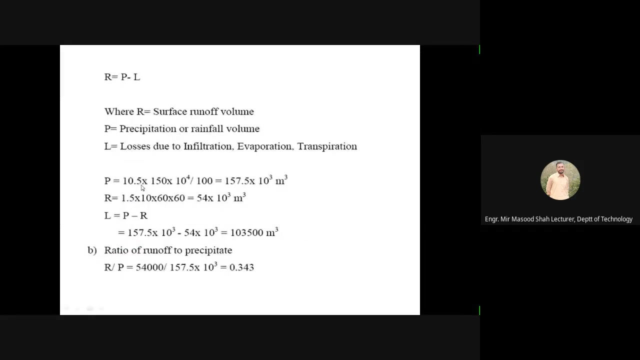